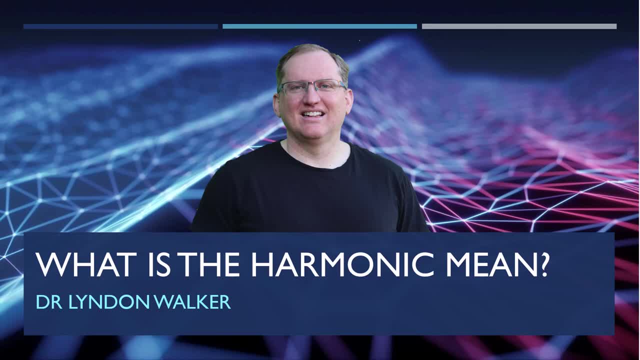 Hi friends, Today I wanted to do a short video talking about the harmonic mean. So the harmonic mean is different from the arithmetic mean, the one that is most common, where we add up all the numbers divided by how many there are, and also different from probably the second most common. 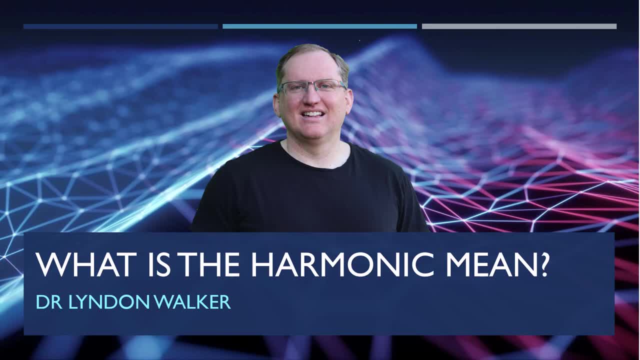 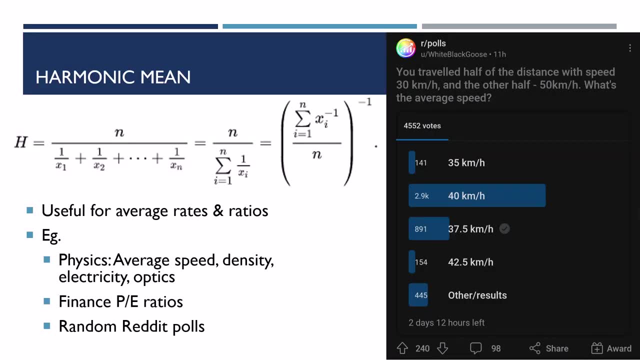 which is the geometric mean where we multiply the numbers and take the nth root. So the harmonic mean has come up recently with some amount of arguing on reddit. So in the data science subreddit there was discussion around this particular question here. So you've traveled half the 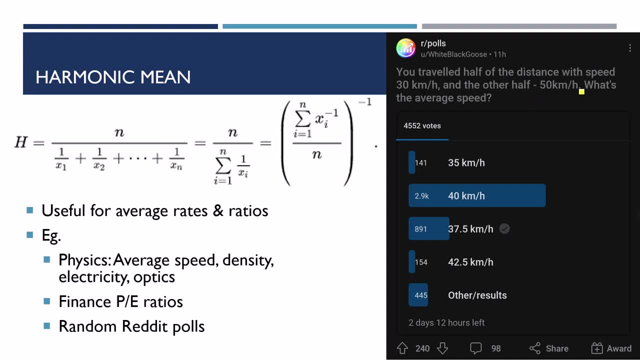 distance with speed 30k's an hour, the other half 50k's an hour. what's the average speed? And we can see that most people answered 40k's and in fact, the correct answer is 37.5.. And the key here is you have traveled half the distance rather than half of the time. 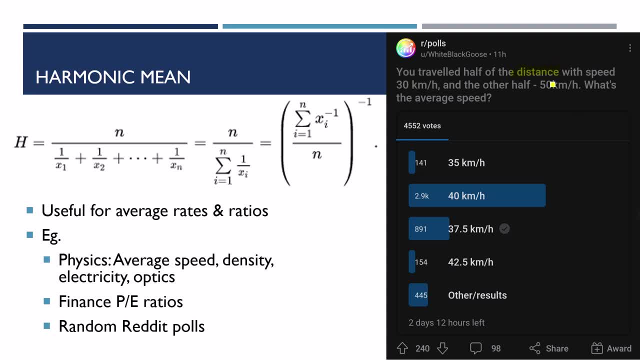 So we're not just taking the midpoint of 30 and 50. And the way that we can do this is by taking the midpoint of 30 and 50. And the way that we can do this is by doing this, And in fact we can do it two different ways, But one of the ways we can do it is with 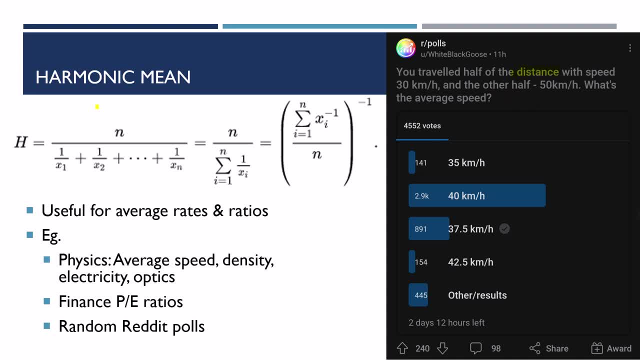 this thing called the harmonic mean. So the harmonic mean is where we take our n, so how many observations? and we divide that by the sum of one over each of the observations. This does require the observations to be positive and definitely cannot be zero. And we can actually turn this if 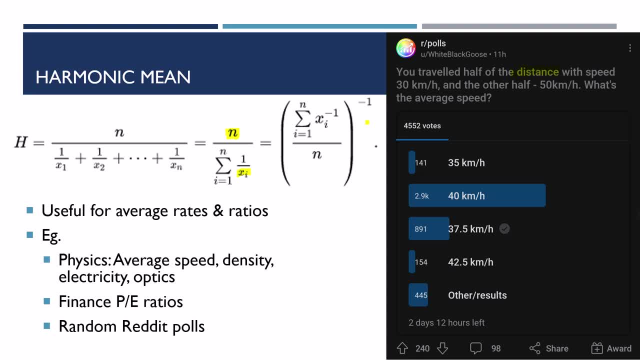 we want into something that we can do with the harmonic mean. So we can do this by dividing it by the sum of one over each of the observations. This does require the observations to be positive and definitely cannot be zero. And we can do this by dividing it by the sum of one over each of the optimisations. This does require 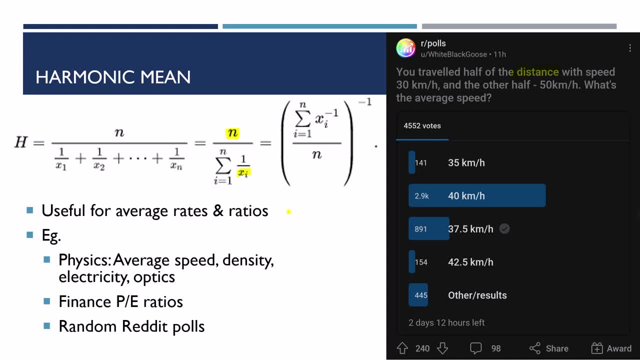 the ratios don't have the same denominators, and so this comes up in physics, and so average speed, which we've seen- this reddit example- is one, and then there's a few others: density, electricity, optics and finance. we have pe ratios, and if we're wanting to get average pe ratios- the price and the 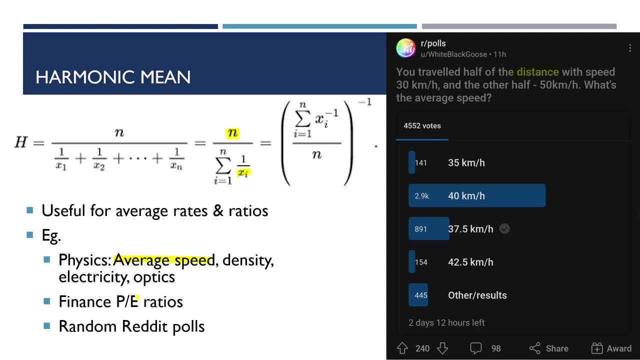 earnings are not always going to be dividing by that same earnings denominator and i guess, technically, the last place where we see it is random reddit polls and threads. if you want to learn more about it, the wikipedia page for harmonic mean is actually pretty good, pretty detailed. if you want to get more technical than this, there's a little bit more of the technical. 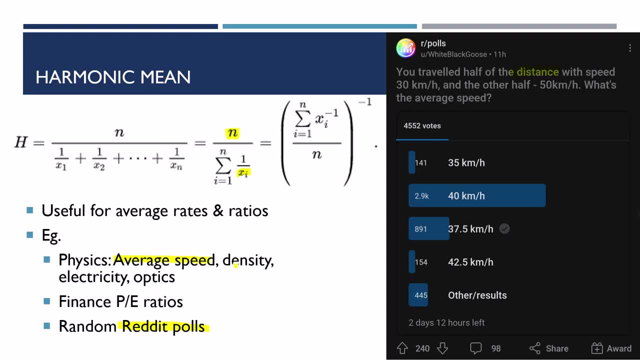 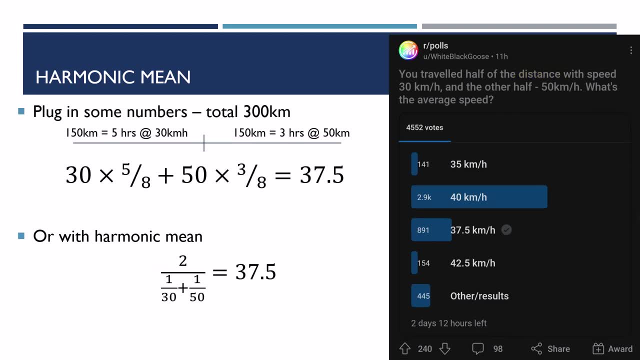 if you want to see slightly more in-depth explanation about these examples. it's got more of that as well, but let's take this question and let's solve it. we're going to solve it two different ways, and so the first thing we're going to do is solve it. 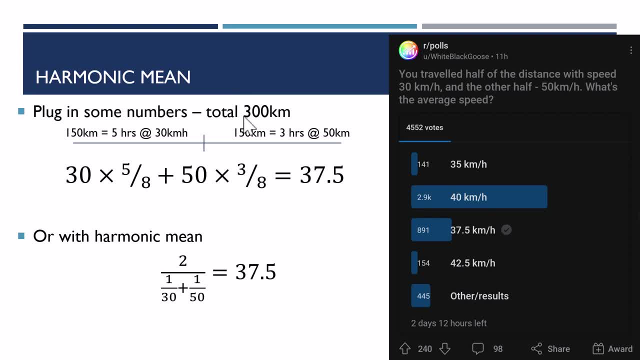 not with the harmonic mean. so we're going to plug in some numbers and we're going to keep it nice and round. so let's suppose we had 300k's the question. they didn't actually give us a number. but 300 is nice because when we split it into half the distance and half the distance, 150 and 150. 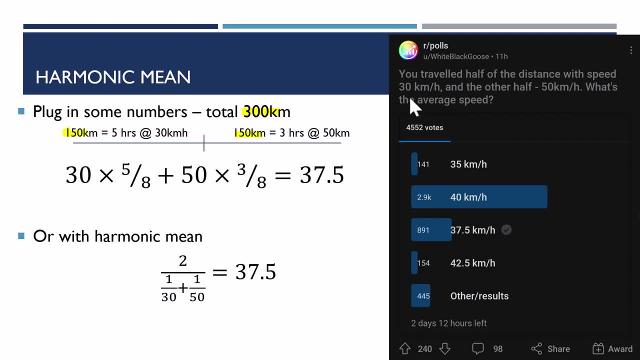 each of those divides nicely by 30 and by 50, so we have five hours traveling at 30 kilometers an hour, we have three hours traveling at 50k's an hour, and so this is where people were making their decisions, and so we're going to plug in some numbers and we're going to keep it nice and 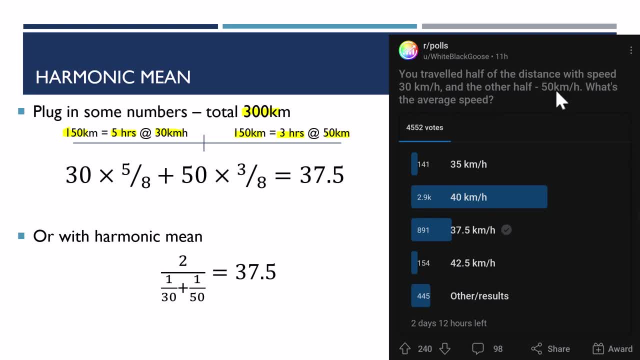 this mistake of assuming they spend half the time at 30 and half the time at 50. in fact, that is not the weighting. so the weighting is five-eighths of the time at 30, three-eighths of the time at 50, and if we work that out then we get 37 and a half. so instead, what we could do is we could use the. 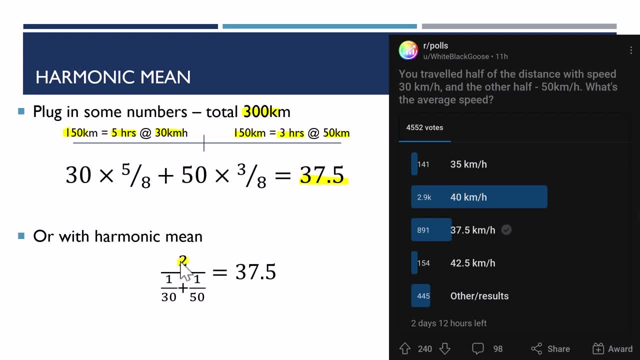 harmonic mean here. so we've got two numbers, two on the top, on the bottom, one over 30 plus one over 50. we compute that and we find that we also get 37 and a half. so this is where this discussion of the harmonic mean came up, and certainly we can solve this question without that and, in fact, i think, intuitively most. 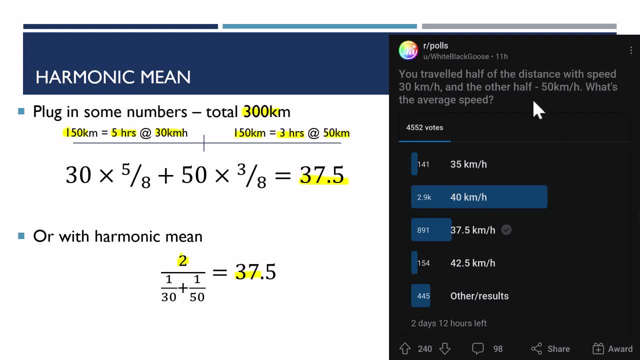 people would and probably even most people should, but it does highlight that whenever we're talking about ratios, really important to be thinking about denominators in our ratios. so what are we scaling? what are the figures out of? and in the case of this, which apparently was in a job interview, i